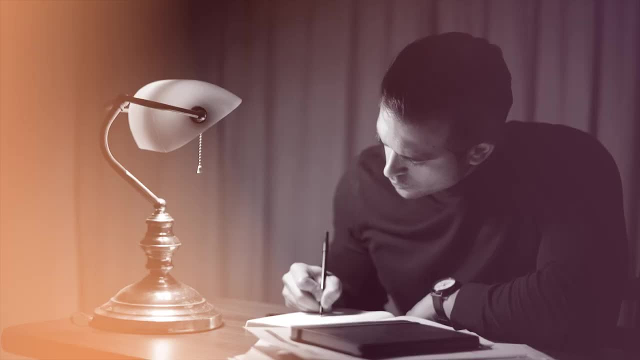 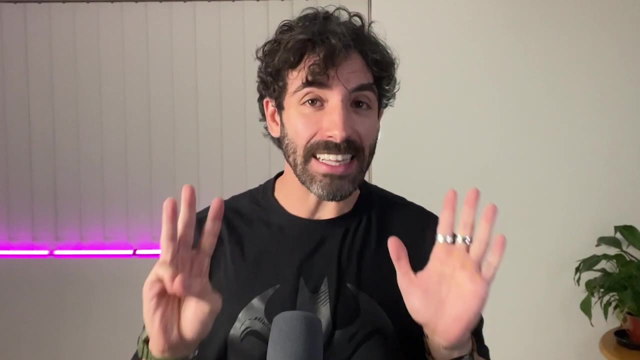 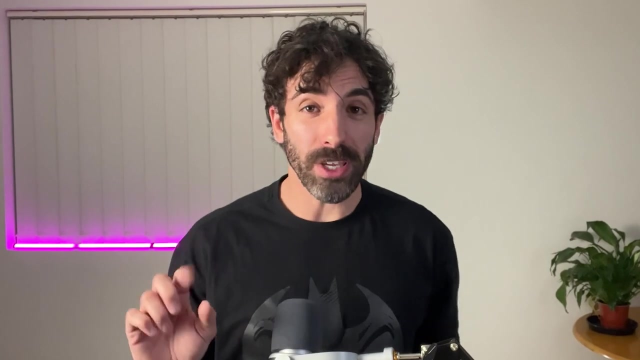 Today's video is all about optimizing your life as a civil structural engineer. Whether you're just starting out or you've been in the game for a while, these eight simple tricks are sure to make your professional and personal life a whole lot smoother. The first trick we're going to go over. 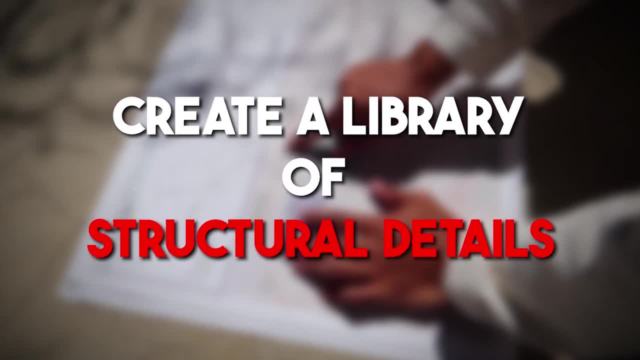 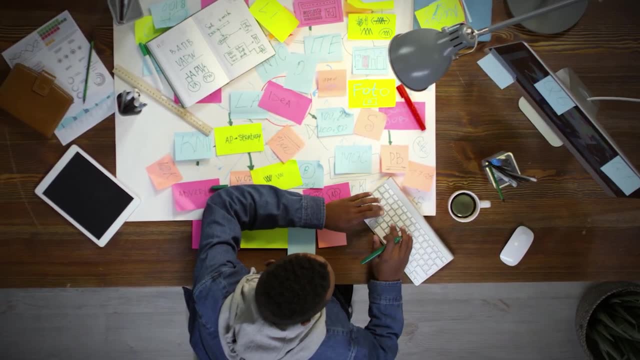 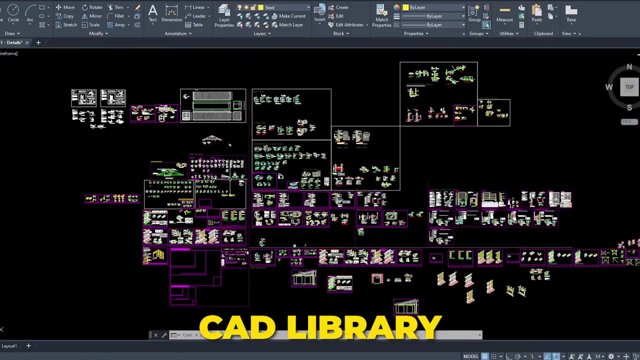 is to create your own library of structural details. Having a go-to library can save you tons of time and streamline your workflow, And here's a quick step-by-step guide to help you create your own library. Step one: head over to your CAD library and PDF the details you use. the 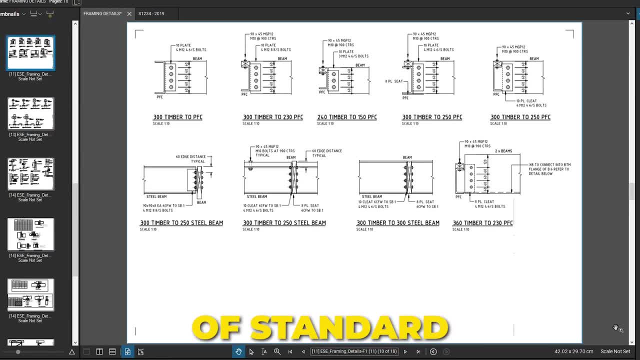 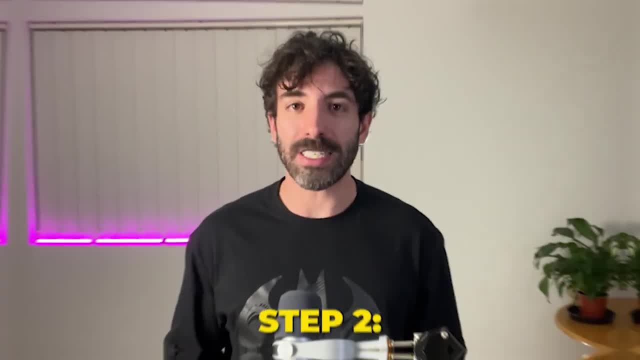 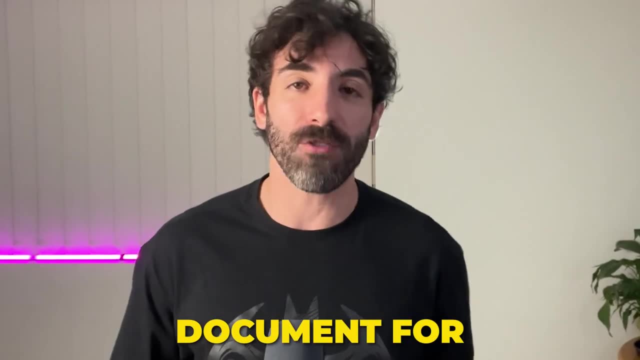 most. This ensures that you have a collection of standard details ready to copy and paste into your structural markups, saving you valuable time. Step number two: organize these details into separate documents and categorize them. For example, a document for framing details, another for footing details. reinforced concrete connections. 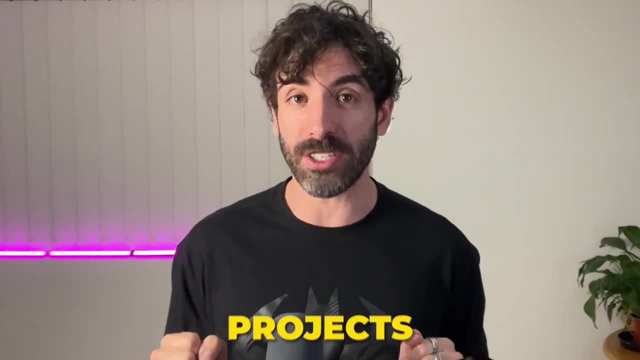 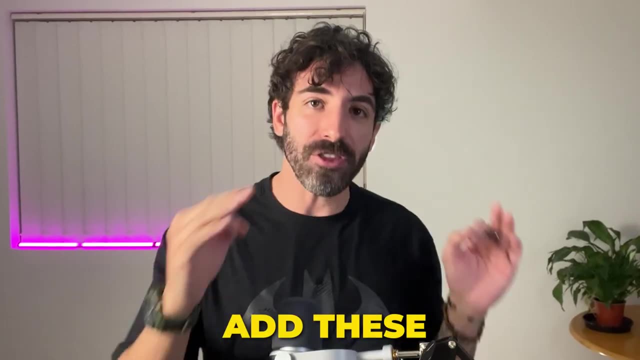 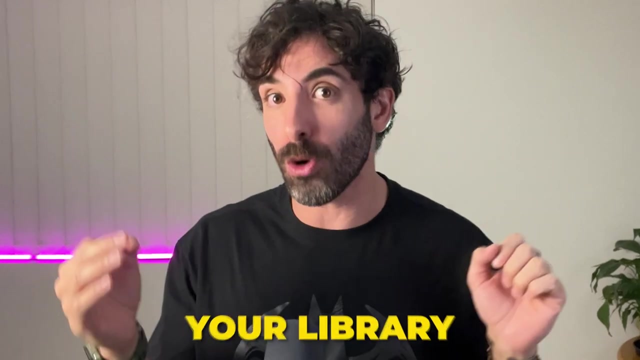 and any other categories relevant to your typical projects. Step number three: research for interesting details from past jobs that could be useful again. Add these to your library, and also snip details from other engineers you come across and add them to your library as well. Step number four: keep this PDF easily accessible for new projects. Use it and. 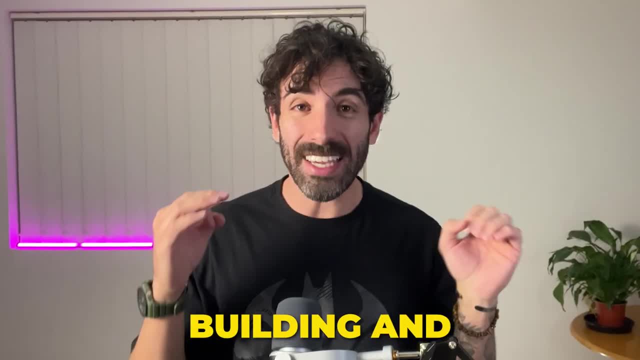 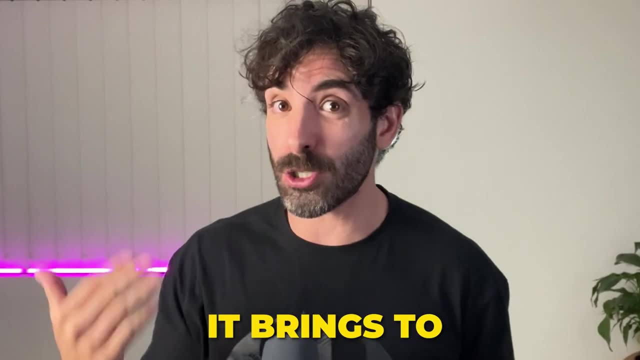 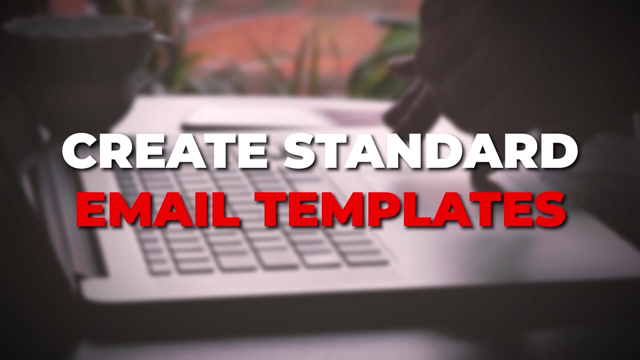 keep adding details to expand your library. Building and maintaining a go-to library might seem like a small task, but the time and workflow efficiency it brings to your projects are immeasurable. Moving on to the second trick, creating standard email templates, This can be a game changer when it comes to handling recurring messages efficiently. 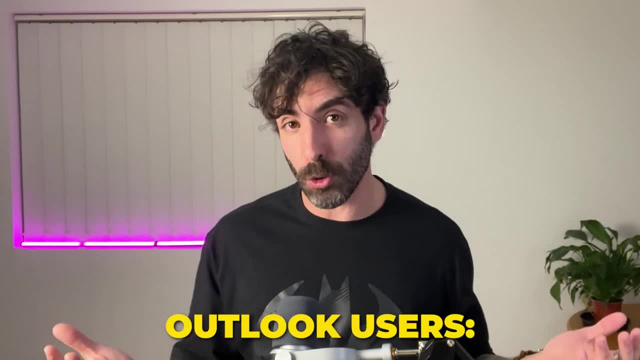 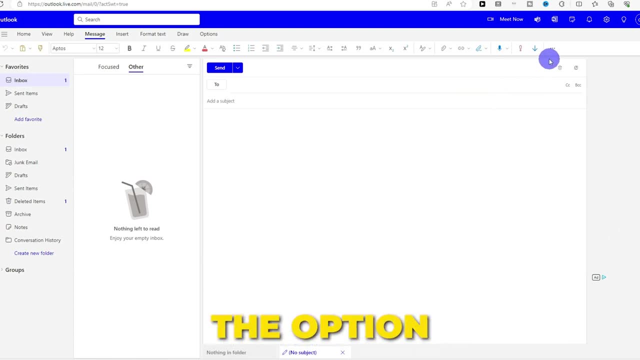 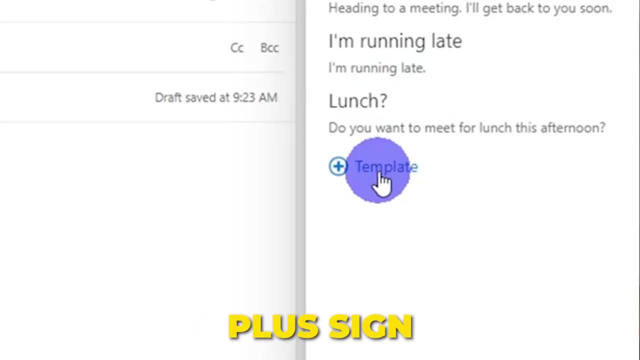 Here's a step-by-step guide, particularly for Outlook users. Open your Outlook email and navigate to the message tab. Within the message tab, look for the option labeled My Templates. Click on it to access your template management. Click on the plus sign or any similar. 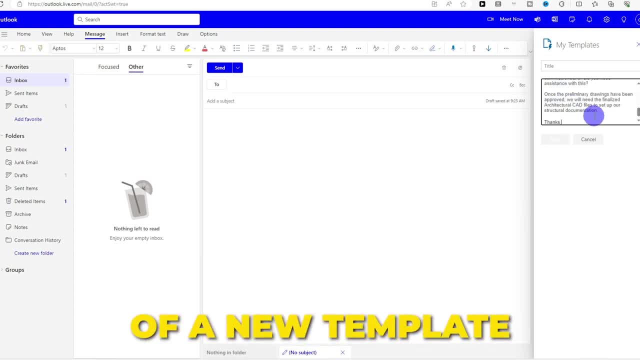 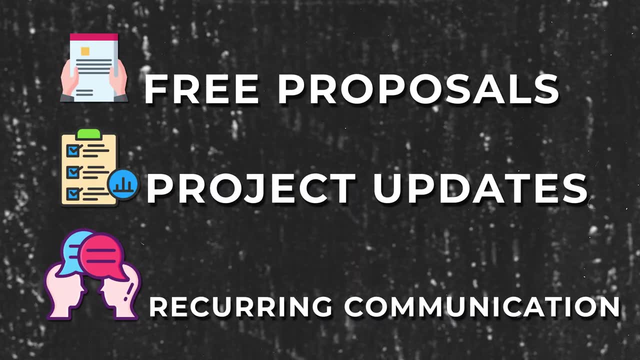 option indicating the creation of a new template. Write the content of the email message that you often find yourself sending repeatedly. This could include responses to fee proposals, project updates or any other recurring communication. Once you've composed the message, you can create your own email template. You can also create your own email template. 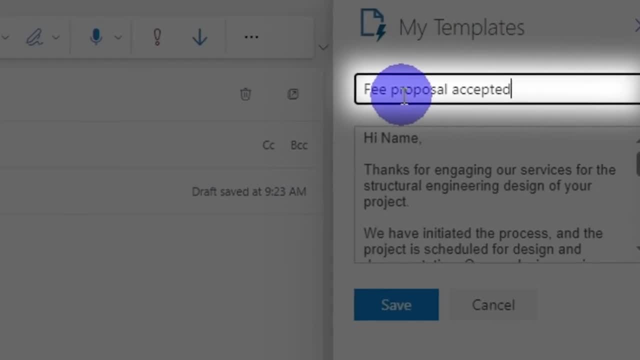 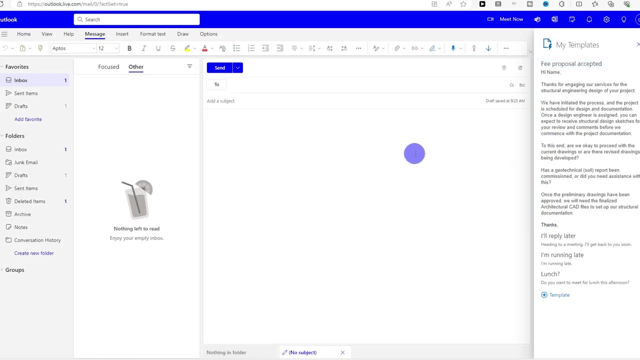 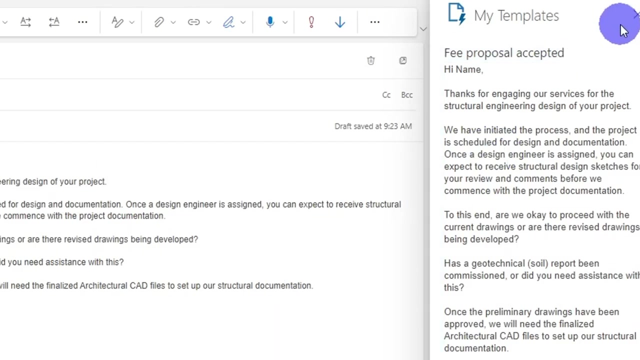 with a name that clearly identifies its purpose, making it easy for you to locate later and save it as a template. Now, whenever you're composing an email and need to send a standard message, simply go to My Templates. select the appropriate template. 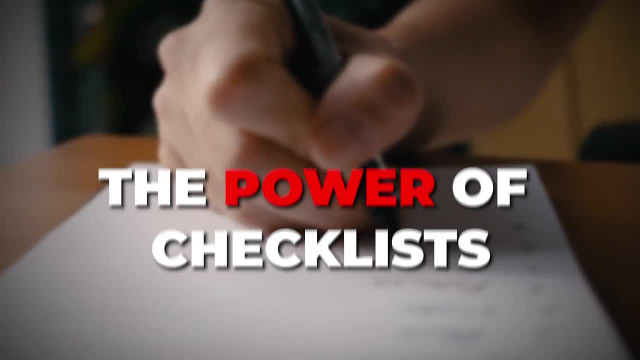 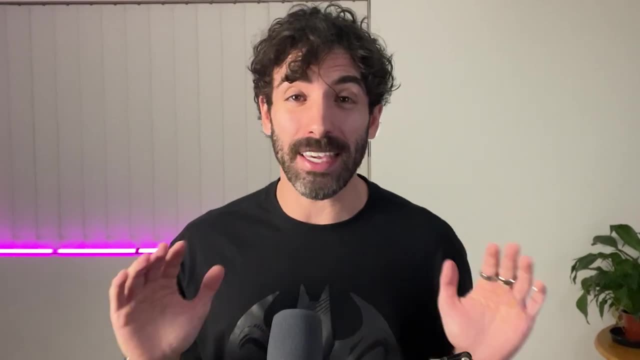 and voila, your message is ready to go. Now let's talk about the power of creating checklists, A simple yet incredibly effective trick that can make a huge difference in your work as a structural engineer. In my previous video- Six Lessons from Six Years as a Structural- 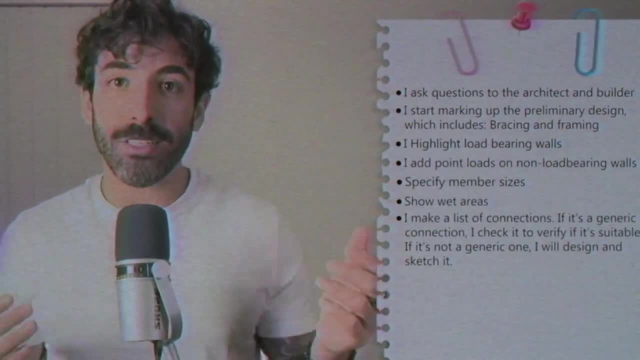 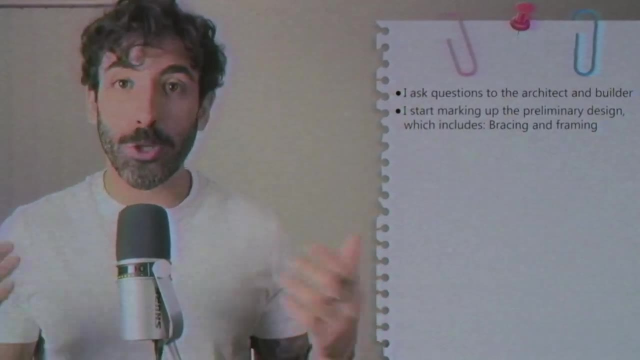 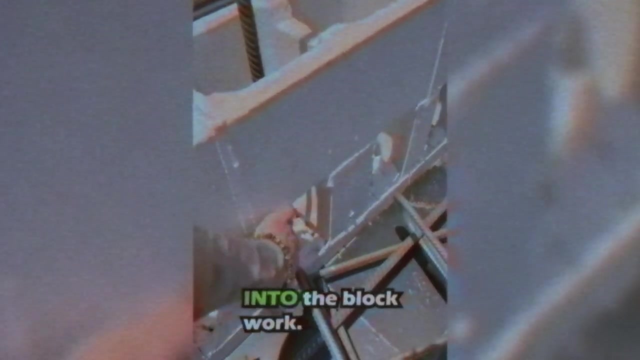 Engineer, I shared a condensed roadmap for designing a house. While designing a house involves many details, I distilled the most crucial points into a convenient checklist format so I don't miss anything Likewise in another video of mine. Structural Inspections- Tasks You. 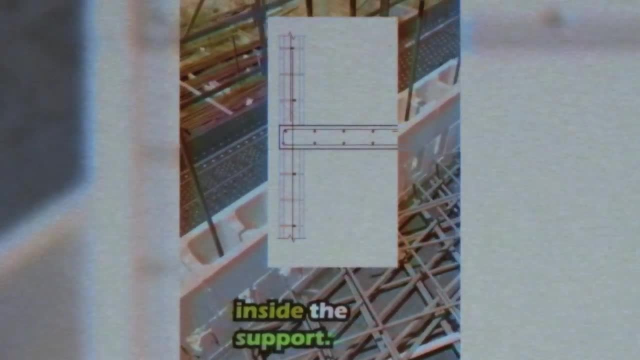 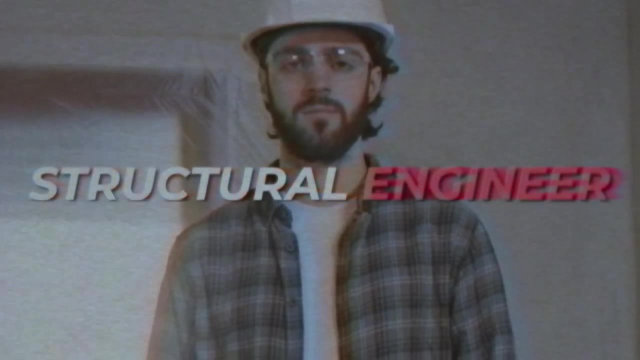 Should Never Miss. I've provided a comprehensive checklist covering the following topics. I've also provided a checklist covering critical aspects in the structural inspection of footings, columns, walls, suspended slabs, steelwork and timber framing. This checklist acts as a reliable guide. 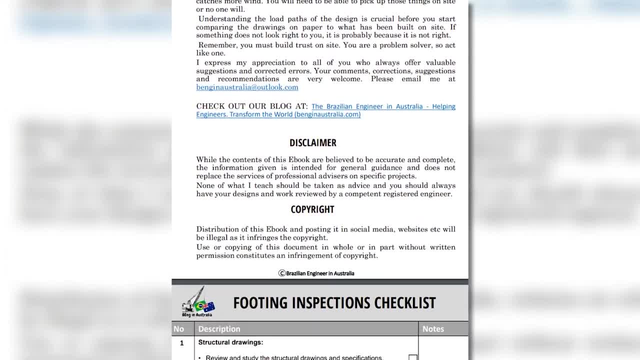 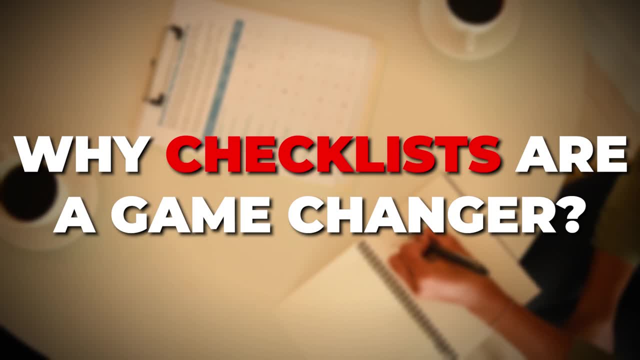 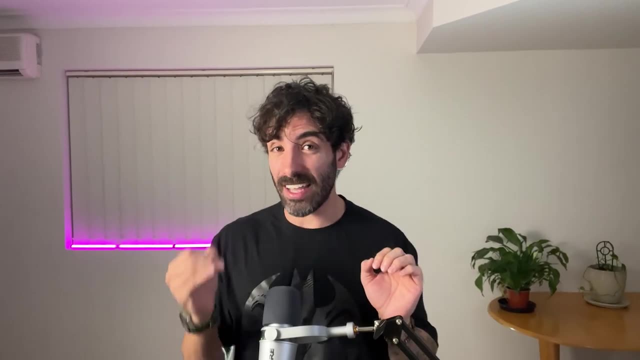 during structural inspections, ensuring that no vital element is overlooked. You can get this checklist for free in the description of this video. So why are checklists such a game-changer for us as structural engineers? I think the main point is that they prevent. 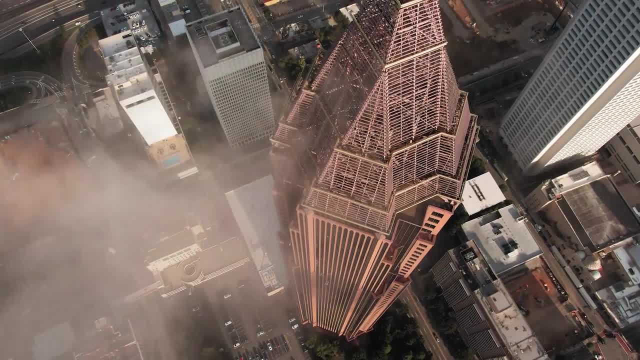 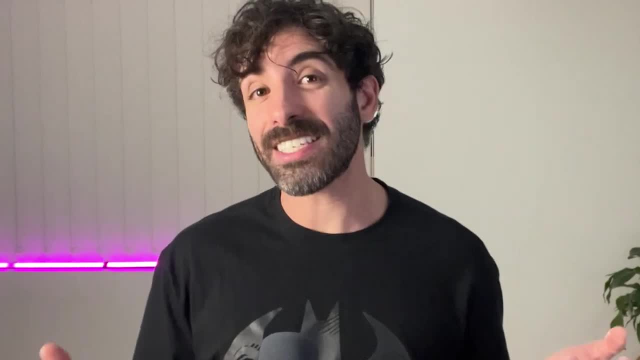 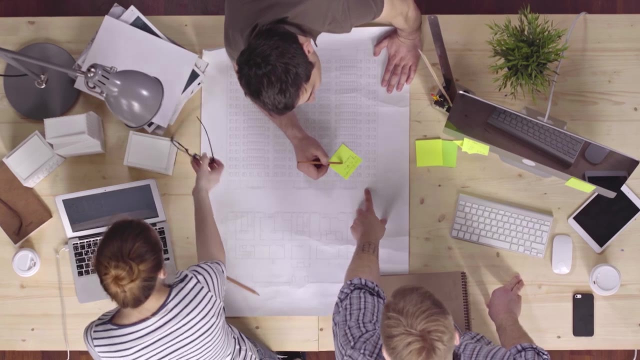 oversights. The nature of all work demands meticulous attention to detail, so having a checklist for every typical activity you engage in acts as a safety net, helping you avoid oversights, Not to mention that they are a great quick reference guide and help you maintain consistency. 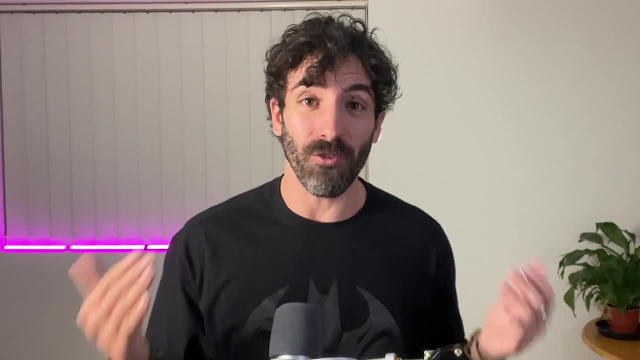 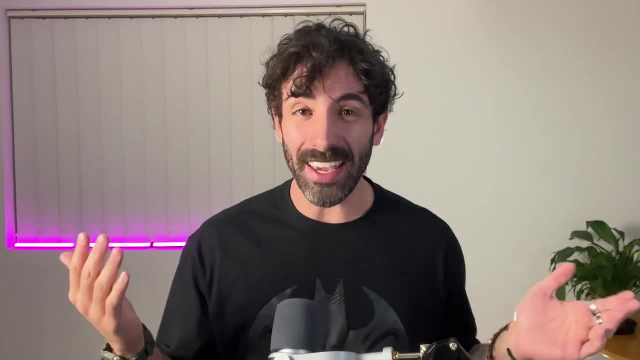 and standardization. Trick number four: lessons learned folder. I have a special folder called lessons learned for each company I've worked before. Whenever I'm making a mistake or learn something new, I write it down. This helps me remember what went wrong. 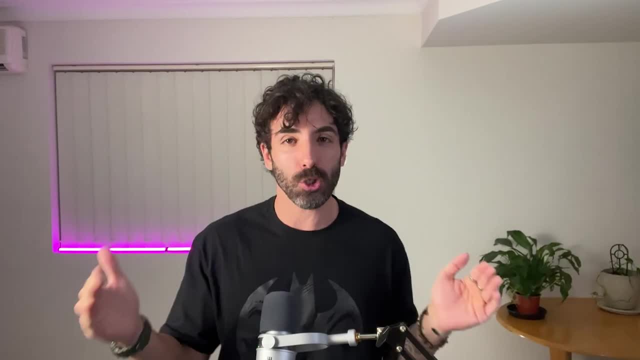 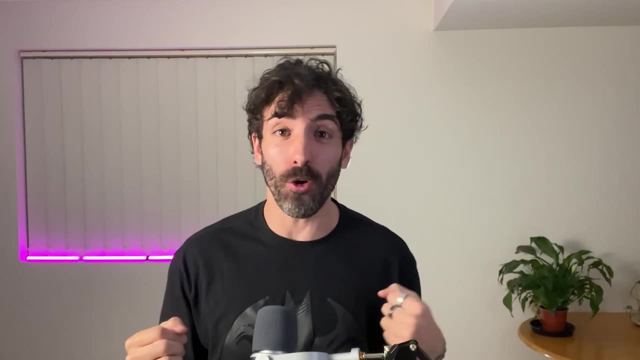 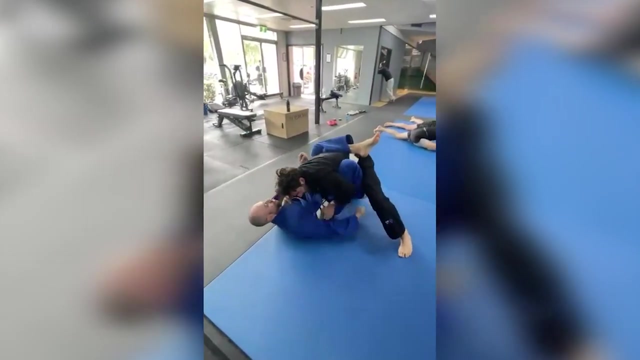 so I can avoid repeating those mistakes and keeps track of all the cool things I've learned. And I don't just do this for work. I also have a lessons learned folder for my jiu-jitsu classes. If I learn a new move or get smashed by someone, I jot down different ways. I could have done it better. 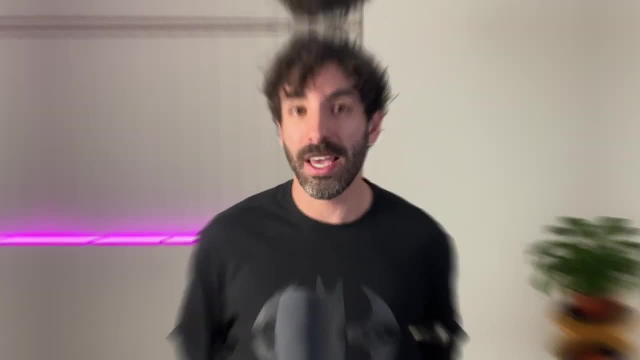 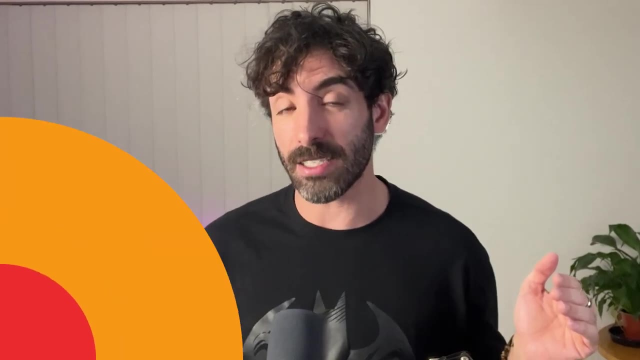 I even have a lessons learned folder for my relationships. If I mess up with a friend or a family member, putting it down on paper helps me learn from my mistakes. Think of it as your very own guidebook, sort of like keeping a diary, So by writing down. 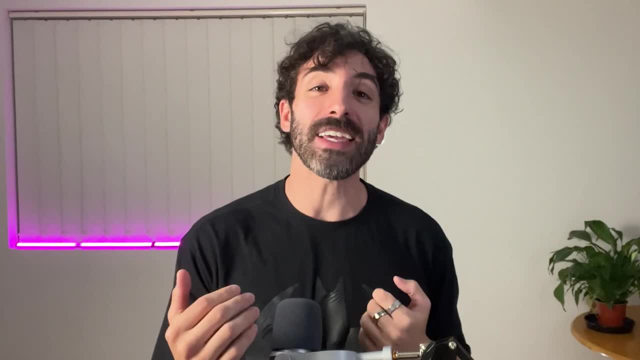 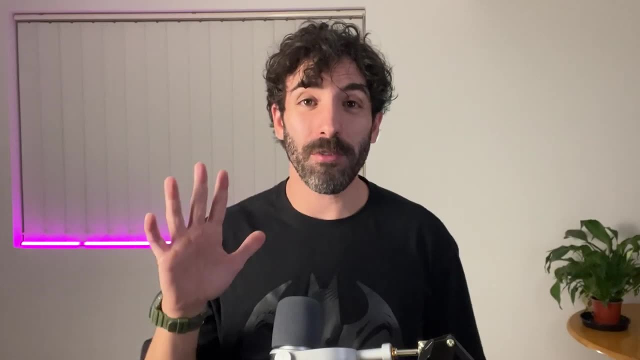 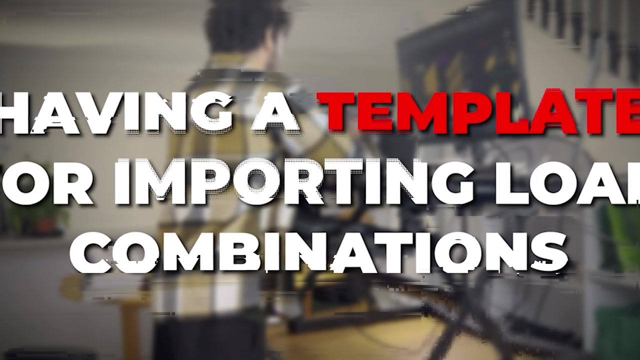 the things that go well and the ones that don't. you create a super helpful guide that helps you become a better person, which makes you a better engineer. Trick number five is all about having a template for importing load combinations into your structural analysis software. 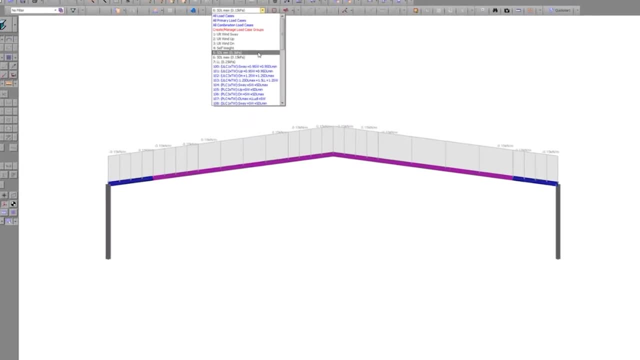 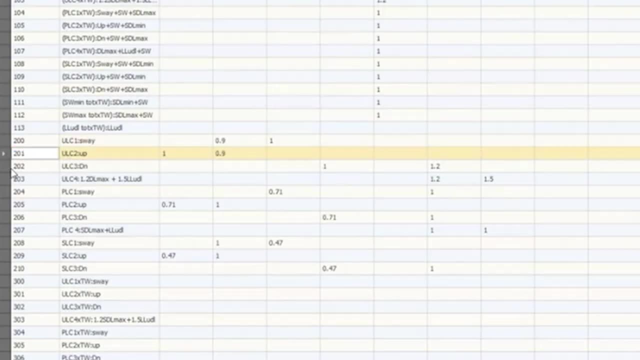 This smart practice can save you from the repetitive task of entering the same inputs over and over again. Setting up templates is especially handy for complex structures like portal frames, where numerous combinations need to be checked, as we've shown in our space gas workshop. 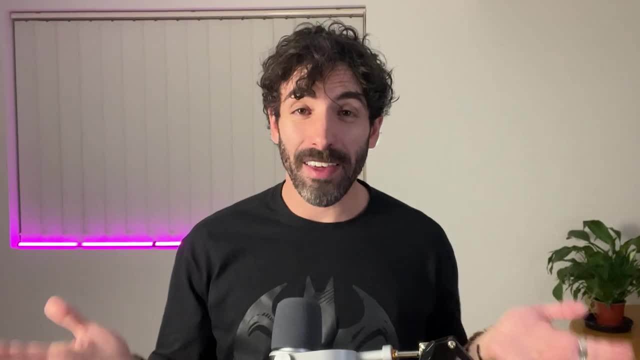 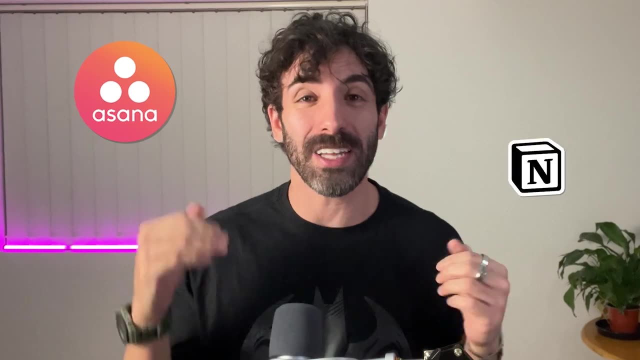 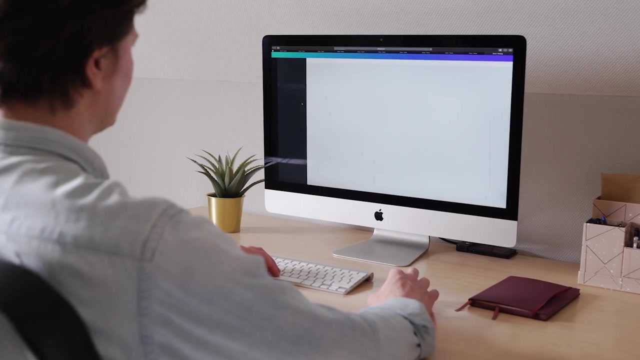 Trick number six: decluttering for clarity. Decluttering is a powerful approach to enhance clarity and productivity. Starting up on productivity apps, embrace the idea that less is more. Begin by organizing your digital environment. Maintain a clean desktop on your computer, phone and iPad. Take a look at my 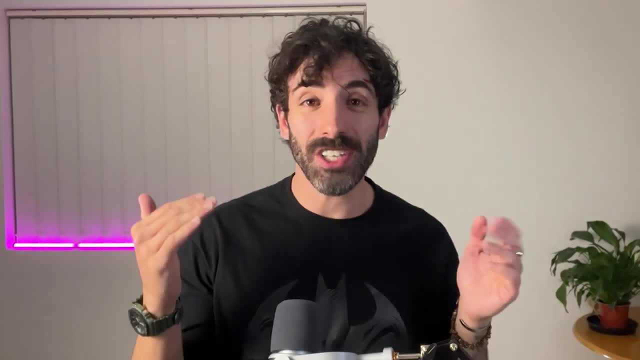 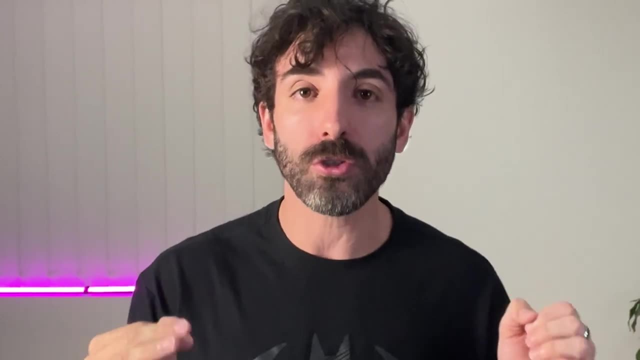 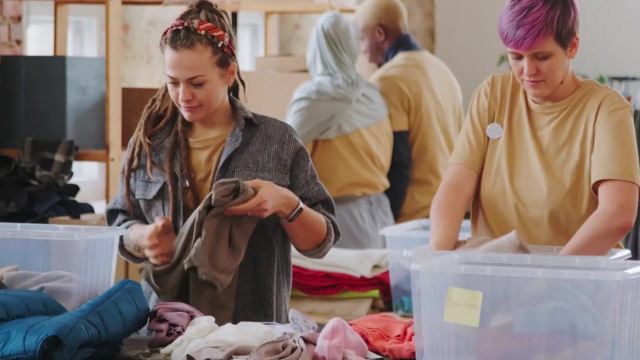 desktop, I only keep the essentials. Extend this decluttering mindset to your physical spaces. Keep your workplace and desk neat for a more focused working environment. The same goes for your wardrobe. If choosing what you wear is too long, it might be time to donate some clothes. Remember, a clutter-free space equals. 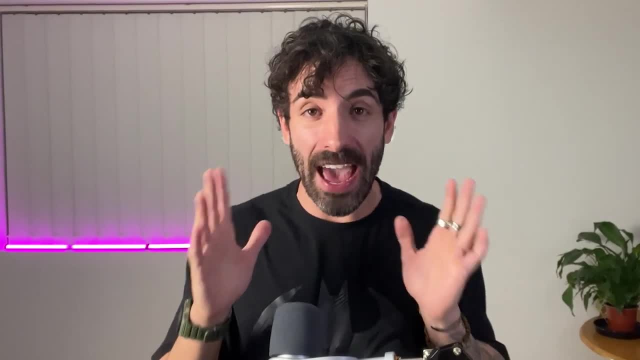 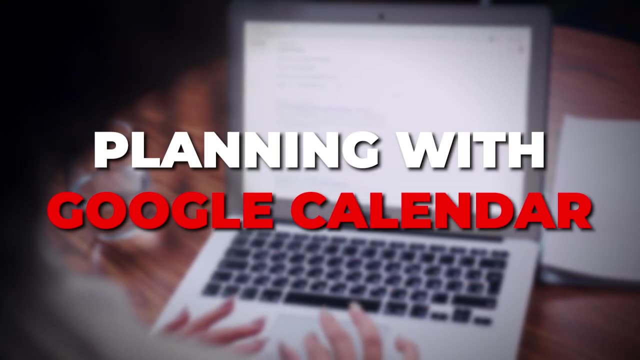 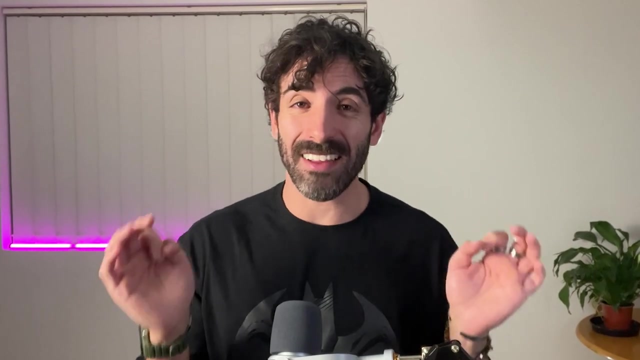 a clear mind. It's a simple yet impactful trick to maintain focus and efficiency in your professional and personal life. Trick number seven is all about organizing your day and week using Google Calendar and Tasks. Let me tell you, Google Calendar is simple and super easy to use. I literally have my 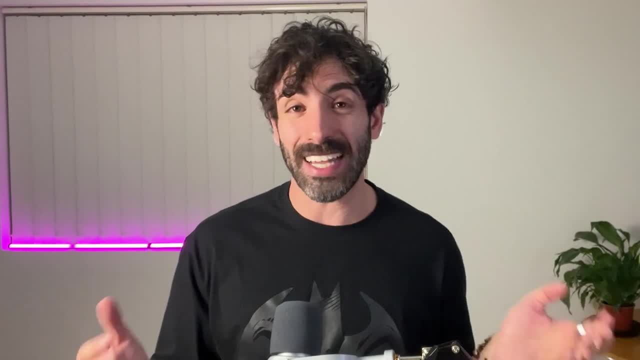 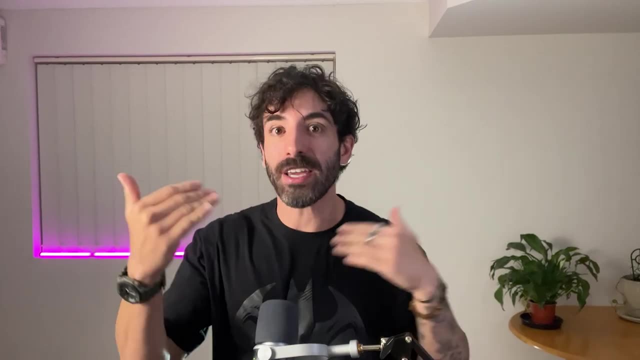 life in my Google Calendar. This brings me so much clarity and helps me avoid procrastination. I don't waste energy trying to remember tasks and I don't spend time figuring out what to do. It's all right there in my schedule. To keep it visually clear, I use two colors.